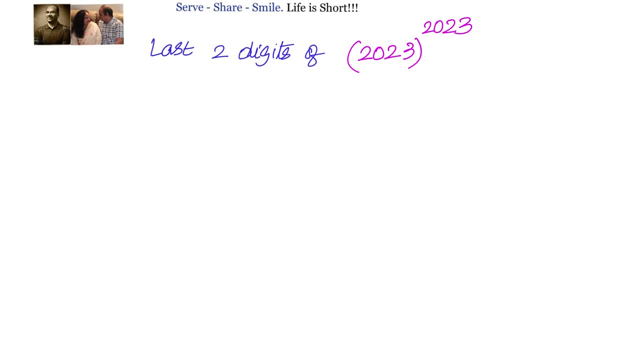 So for that let us have a look at the different powers of 3,, 7, 9 and try to understand. If I take 3, I know 3 power 4 is 81 and I also know that 7 to the power of 4 is 2401.. 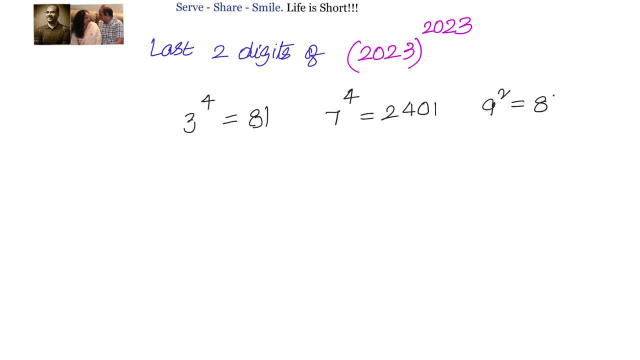 I know 9 square is 81. So basically any number which is ending with 1 or 7 or 9 is 81. So basically any number which is ending with 7 or 9 is 81. So basically any number which is ending with 7 or 9 is 81.. 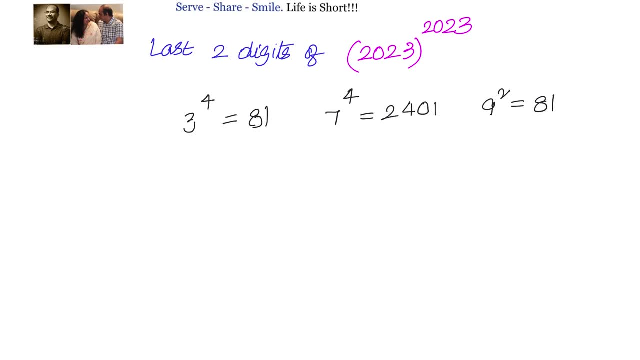 Similarly, any number ending with 3,, if I am able to rise it to the power of 4, it will be ending with 1.. Similarly, 7 rise to the power of 4 and 9 rise to the power of 2.. 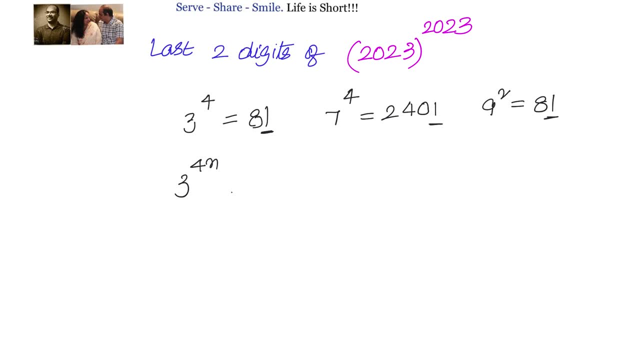 So can I go ahead and say that 3 power 4n, 7 power 4n and 9 power 2n will be ending with unit digit 1.. Now, if that is going to happen, then it is a good news. 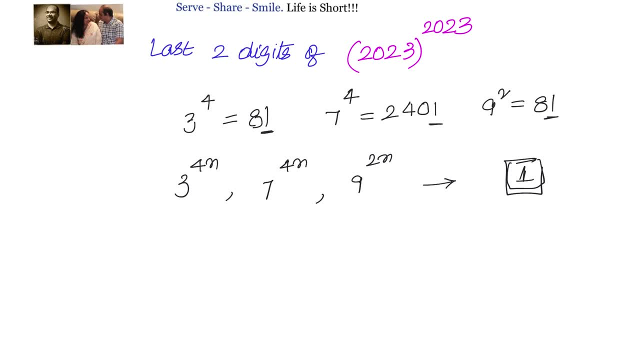 Because we know that, how to deal with the numbers which are ending with unit digit as one. so let's go ahead now, apply this logic and try to find out first what is 2023 whole to the power of 2023, last two digits. so let's let me just write it down so we just now understood that the given number we have to 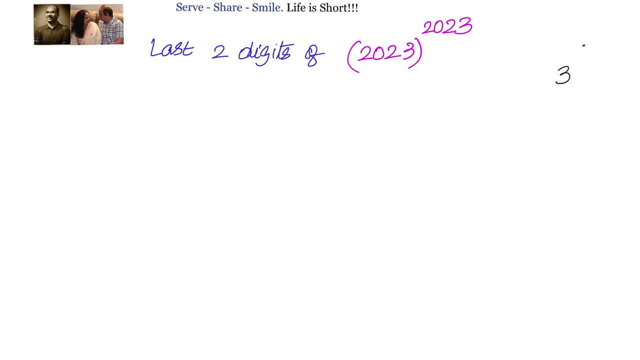 if it is ending with 3, i have to raise it to the power of 4 so that it will become ending with 1. then i have to see: whatever the power, i can easily handle it because i have the number now ending with 1. whatever may be the power, i know the logic, what i need to do so that i can get the last two. 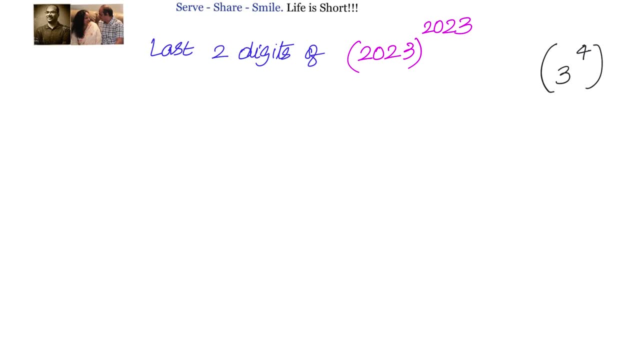 digits. so let us raise this number to 4, for that i will write down: 2023 can be written as 4 in. 4 in 2023 can be written as 4 in 2023 can be written as 4 in 2023 can be written as 4 in. 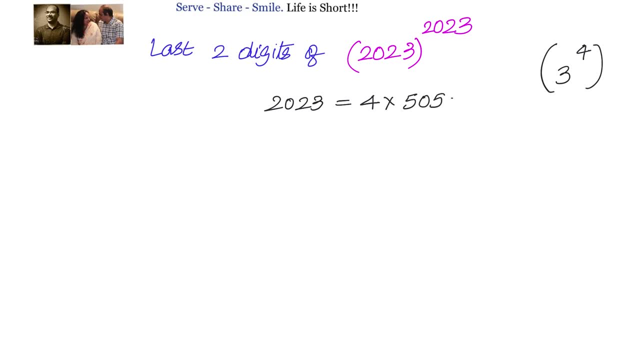 into 505 plus 3. now that logic i am going to apply here and say: 2023 ending with 2023. we are interested in basically the last digit, we are interested in the last two digits. so write it as 2023 whole to the power of 4, because that's what we discussed. we should write down and that: 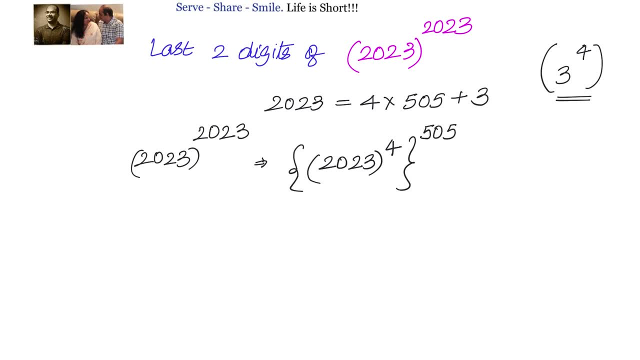 we will raise it to 505 and then we multiply that with 2023 whole to the power of 3 so that we can get 2023 whole to the power of 2023. that's very simple. right 4 into 505 is to 2020 and we are. 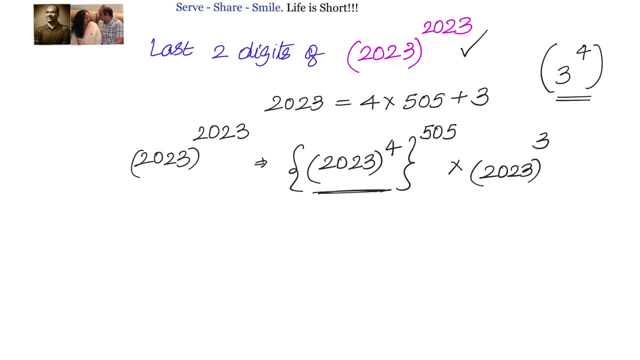 adding three there. now we know this guy is going to end up with one, so let us see what will be the two digits here. i have to multiply 23 four times and i have to take only the last digits. two digits now. 23 into 23 is 529. i will take only the last two. 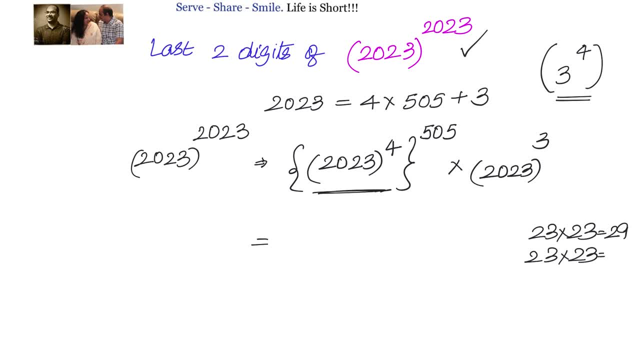 digits. those are 29. again, 23 into 23 is ending with 529. i will take last two digits. these two i will multiply 29 into 29, that will be 841. i'll be taking only the last two digits, so i know that this. 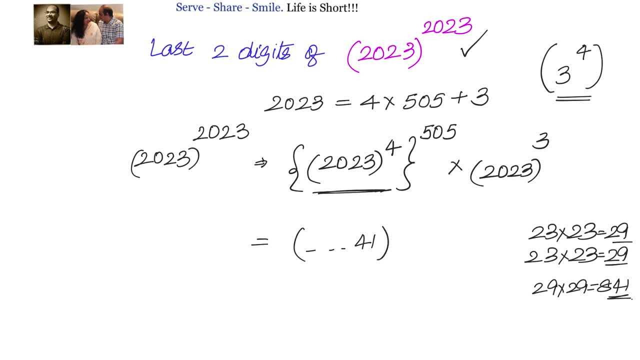 i don't care, but i know it will be ending with four and one to the power of 505, and here we have 2023, whole cube. that means we need to find out the last two digits of this number. 23 into 23, we know, is 29. you multiply 29 with 23 and take only the last. 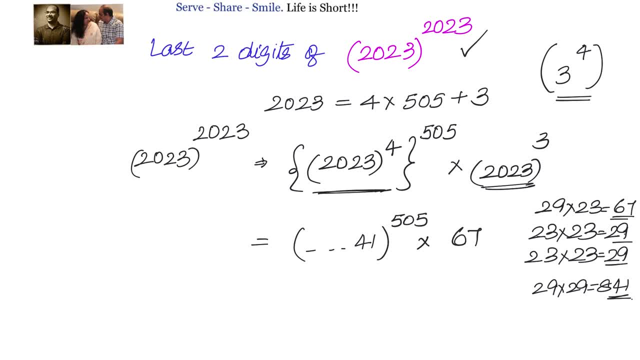 two digits. last two digits are six and seven. now let's go and apply the logic related to numbers ending with one. we know that if you have any number ending with one, so and raise it to any power, the unit digit will be always one, and the tenth digit will be coming from the product of the unit digit in the power multiplied with. 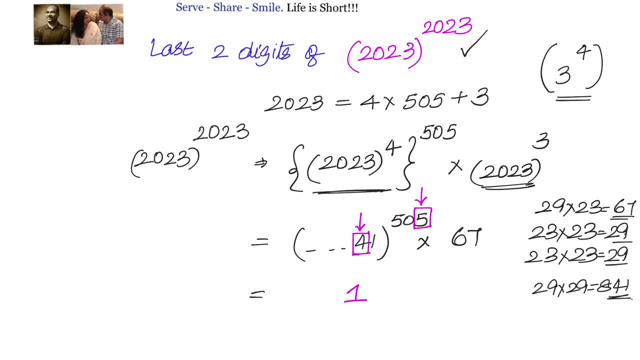 the tenth digit from the number and we multiply this, that is, 4, into 5, 20, and from the 20 we will take only the unit digit. that means it will be zero. now, this we have covered extensively in the earlier video, so if you have any doubts in that, you can just go back to the video where you have. 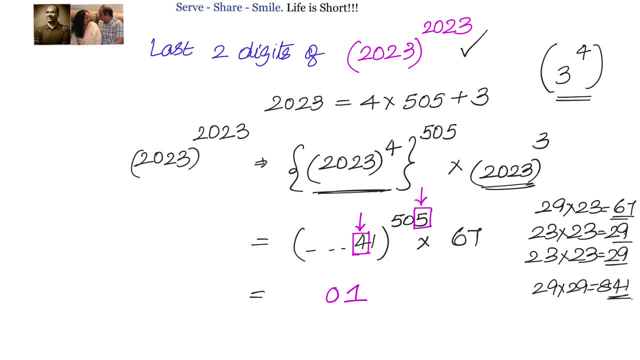 how to find out the numbers ending with unit digit, as one find out the last two digits. now, this is zero one, and that we need to multiply the figure to the last one. uh, and so the fault here, Sau Savage, is v2 won't beONED for the five digits, so we do want to attempt. 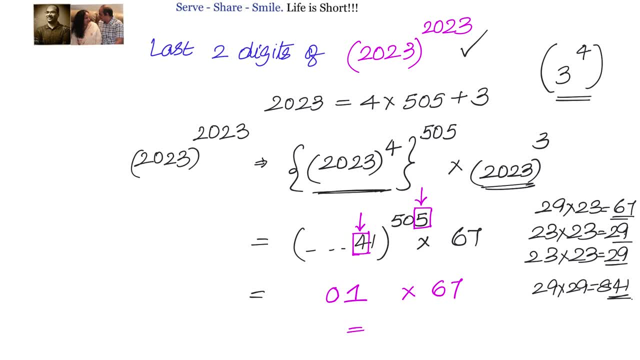 and that we need to multiply with 67, so 1 into 67 is 67, so the last two digits of 2023 whole to the power of 2023 will be 67. let's have a recap of this before we move to some other examples maybe. 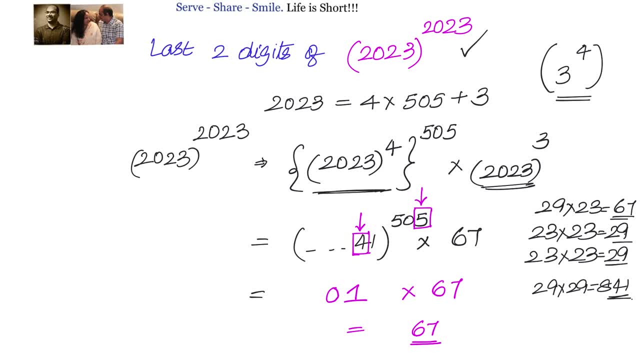 one example for 7 and one example for 9.. 2023 to the power of 2023. we have to find out the last two digits. our logic is to convert the number 2023 into another number in such a way that the number will be ending with 1, so that i can apply the logic related to numbers ending with 1.. so for 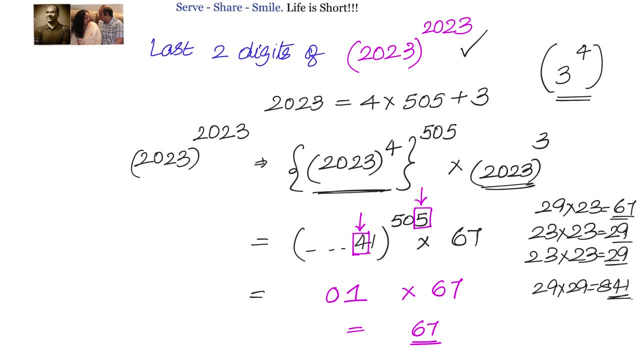 that what we did. we have taken the power 2023 divided with 4, and we understood that can be written as 4 into 505 plus 3, 4 into 500 and 5 plus 3.. now we have went back to 2023, to the power of 2023, and we have written it as 2023 whole. 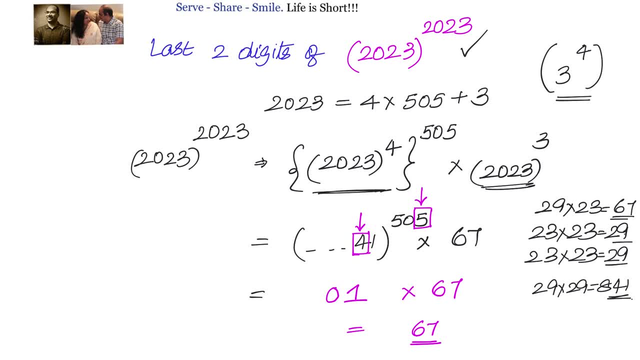 to the power of 4. whole to the power of 505. multiple with 2023: whole cube. now we are going to take only the last two digits. so, whatever the numbers we are multiplying, we are going to take only the last two digits. now check 2023: whole to the power of four. the last two digits will be: coming from 22.000 out of 23.500, which we have taken 2 digit number. the last 2 digits are taken compared to 4, as we see in the shown information. this strength will be less than 12.000 and 3.ism sería. 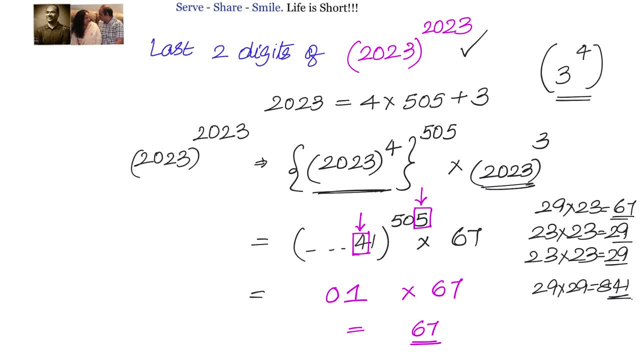 beforehand my last two digits. which is positive value is also stroke former number 3, 0, 5, and that will be multiplying four times. 23 into 23 is 529, but we will take only the 29. similarly, again, 23 into 23 is 529, we will take 29. so 29 into 29 we multiply, we get 841. we will take only the last two digits. 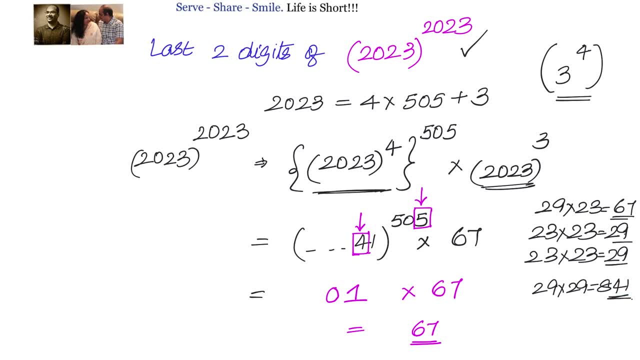 41. now this 41 to the power of 505 we have and that we have to multiply with 23. 2023, whole cube. the last two digits of this number will be ending with 23 into 23 into 23. last two digits: 23 into 23 will end with 29 and 29 into 23 will end with 67. so this whole number will be ending. 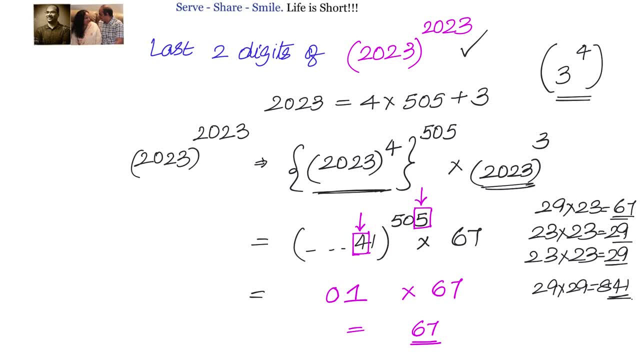 with 67 and now coming to this number- whatever may be this number, but we know it is ending with 41. that is enough for us and we know the power is 505. then the logic is the unit digit will be always one and the tenth digit will be coming from unit digit, from the product of. 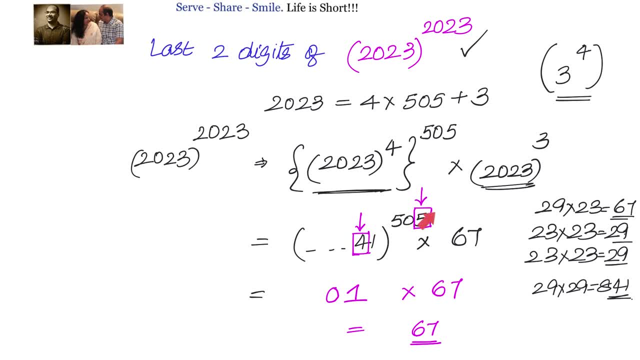 number 5 and number 4, which are unit digit from the power and the tenth digit from the number. so four fives are 20. we are taking unit digit, that is 01. so 2023 whole to the power of 2020 r will be ending with 01 and 2023 whole cube will be ending with 67 when we multiply. 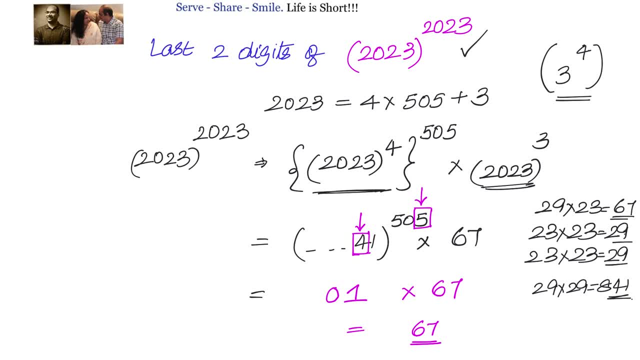 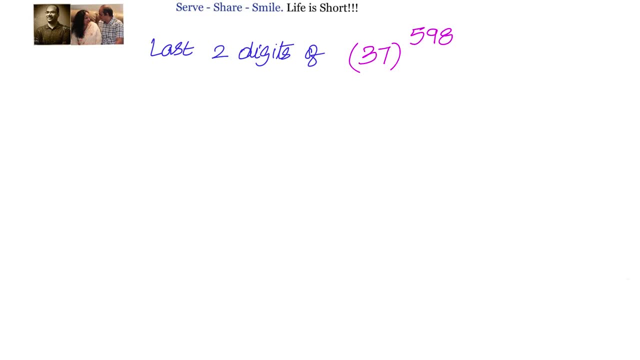 both of them we will be getting that the last two digits will be equals to 67.. Now let's do one simple example related to 7.. Take another example where we have now it is ending with 7.. We know that 7 to the power of 4 will be ending with 1.. So we'll write down 598, the power, as 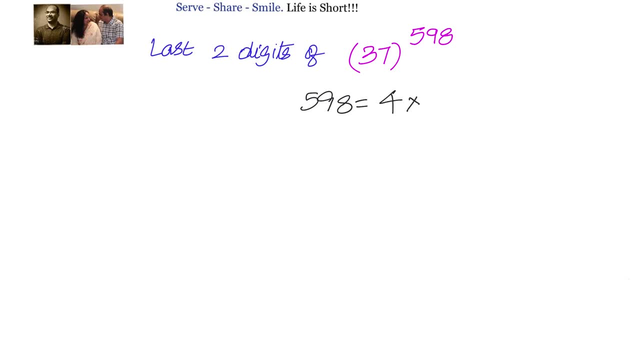 4 into 149 plus 2.. So then we can write down 37 to the power of 599 as 37 to the power of 4 to the power of 149, and that we multiply with 37 square. Now we know that this number will. 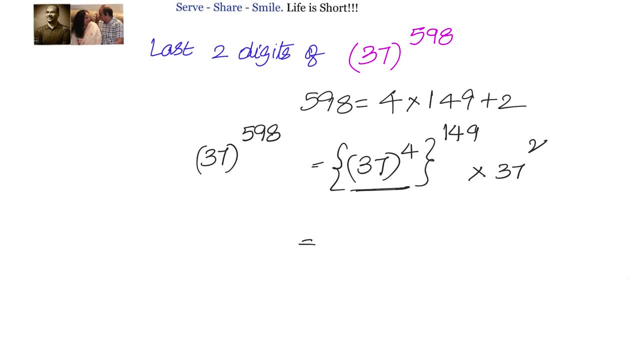 be ending with 1. that will be 37 multiplied four times. so 37 into 37 will be ending with 69 and 69 into 69 will be ending with 61. we are taking only the last two digits, so this will be some number ending with 61 and to the power of 149 multiply with 37 square, we know 37. 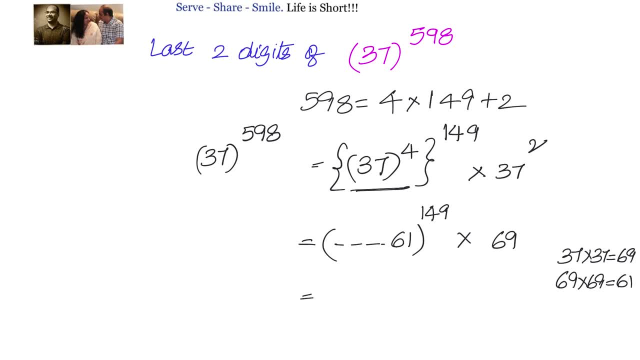 square will end with 69. now 61 to the power of 149. then we know that the unit digit will be 1 and the 10th digit will. the next digit will be coming from unit digit of multiplication of these two numbers, that is, 9 into 6, 54 from 54. we will take the unit digit that is 4, 1, so 37 to the power. 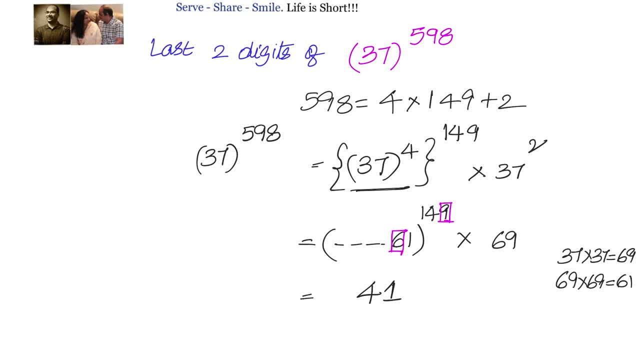 of 4 to the power of 149 will be. last two digits will be 4. 1 that we multiply with 69. again, we need to take the last two digits here. when I multiply 69 into 41, I will be getting 2829, but I will take only the last two. 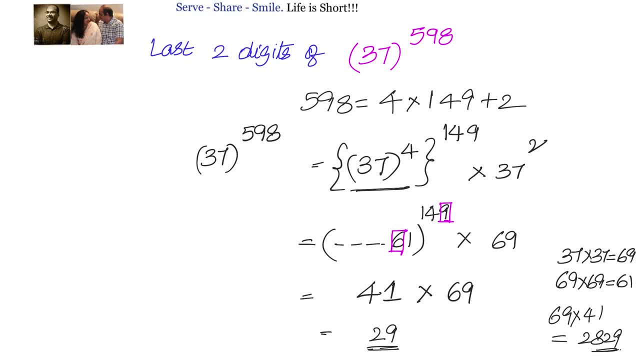 digits. so my answer will be 29. so the last two digits of 37 to the power of 598 is 29. similarly, we will do one example with respect to 9. now let's find out the last two digits of 729 whole to the power of 236. we know. 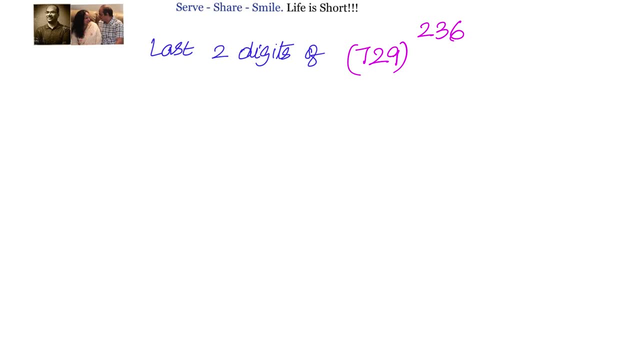 that with respect to nine, we have to make it the number raised to the power of two. so I will write this as 729 whole square, so that the number will end with 1 and what it will become 236. I have to write it as multiple of two, so it will be 2 into. 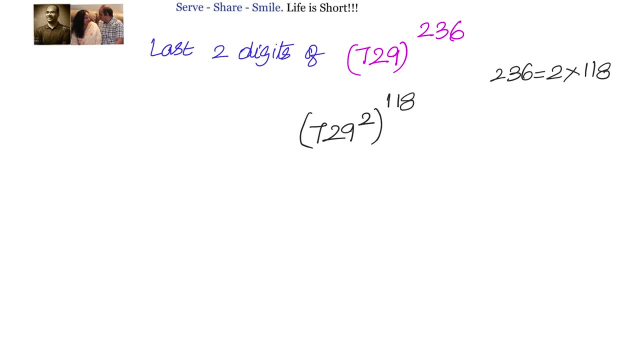 118. so I can write this number: 729 whole square, whole to the power of 118.. We know that 729 square will end with 29. into 29, that is 841.. We'll take only the last two digits, So this number will be ending with 4. 1 to the.